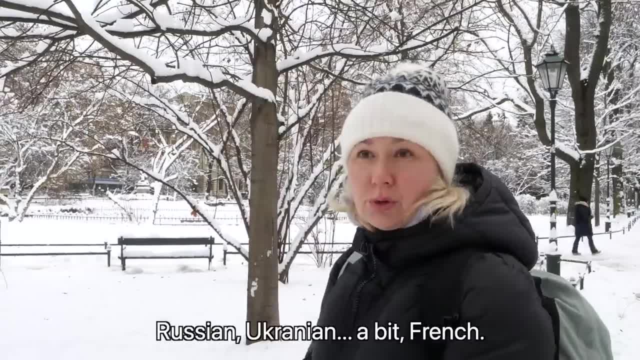 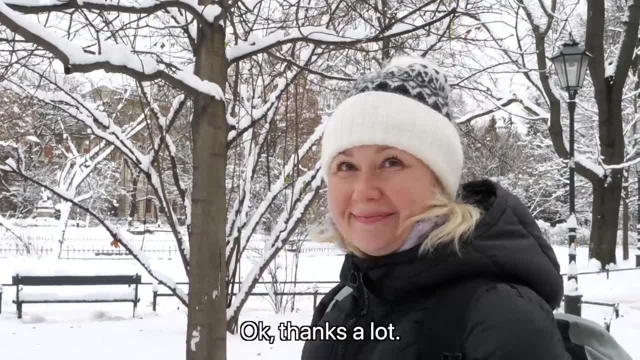 And French, Polish, No, And French, Okay, Thank you very much. Thank you, You're welcome. What I need to say? I just asked- I asked many different people one question. I don't know, I don't know. 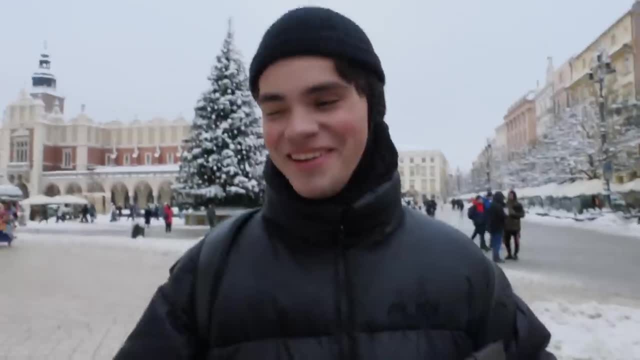 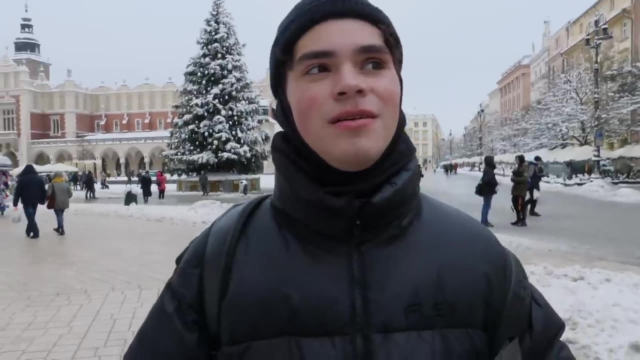 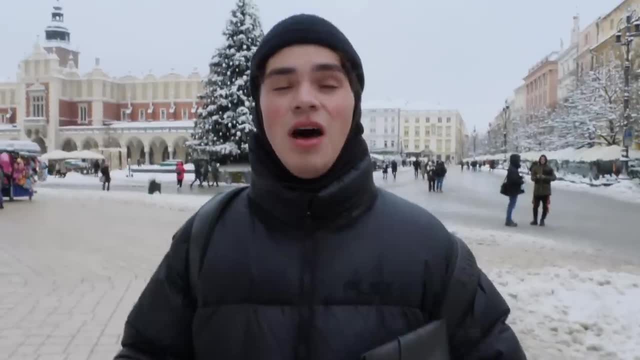 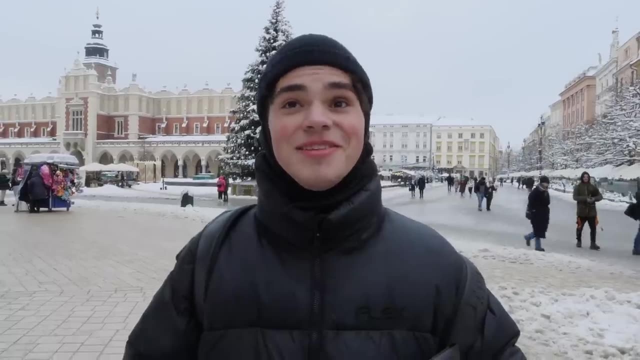 Okay, Yeah. So how many languages do you speak? I speak in four languages, That's Ukrainian language, Russian language, English language and Polish language. Wow, Yeah, And I live in Poland, but I'm from Ukraine, Wow. 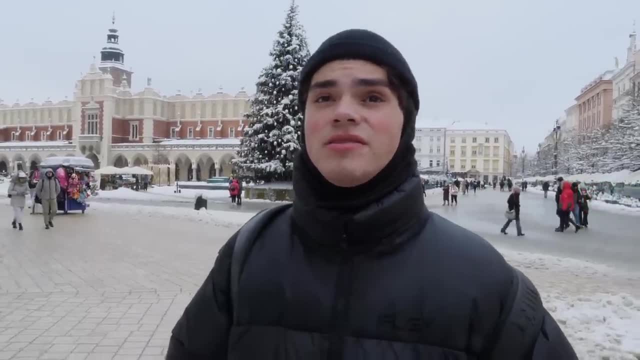 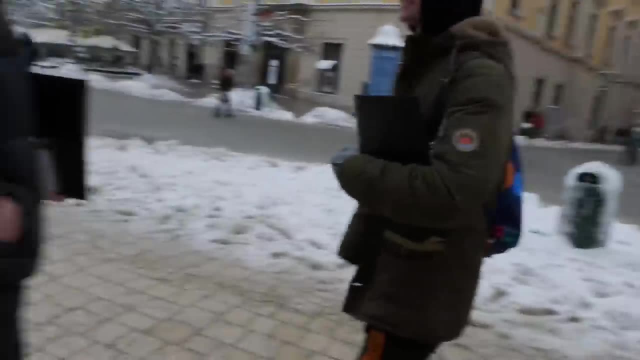 What do you think of Poland from your time there? I think it's a very nice country And Krakow is one of the best city in Poland. for me, That's awesome. Okay, Thank you. You want to answer? No, no, How many? How many English little? 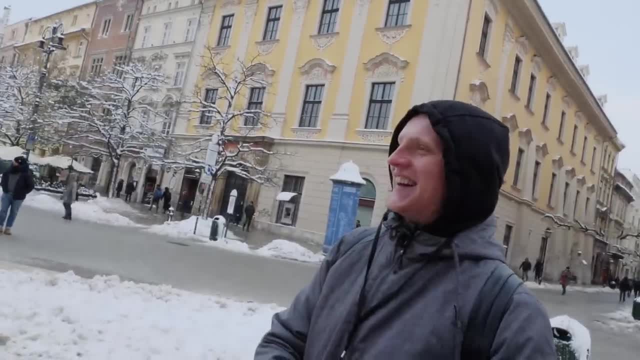 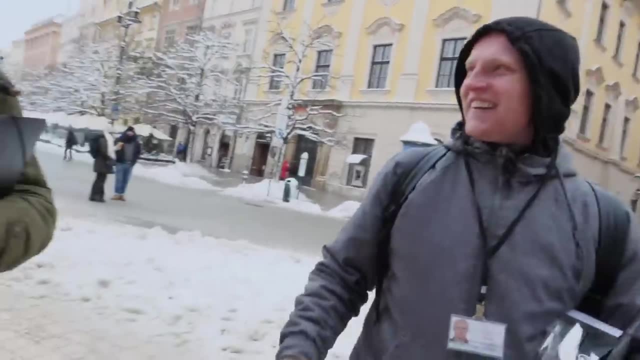 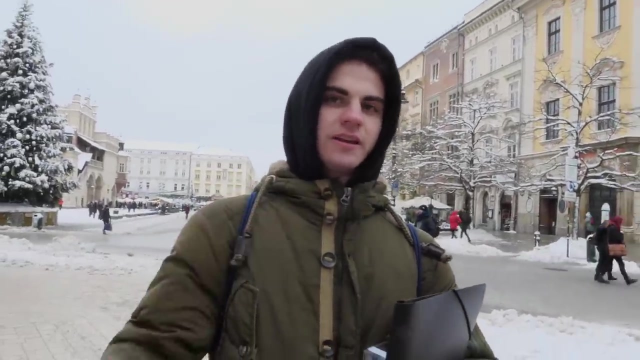 Hello, Ukrainian. Polish English, little English, no, Polish, Yeah, Polish, Polish. I'm from Ukraine, but I can speak Polish, maybe a little bit English. Is it hard to learn Polish, or it is similar to Ukrainian? Similar, Similar. 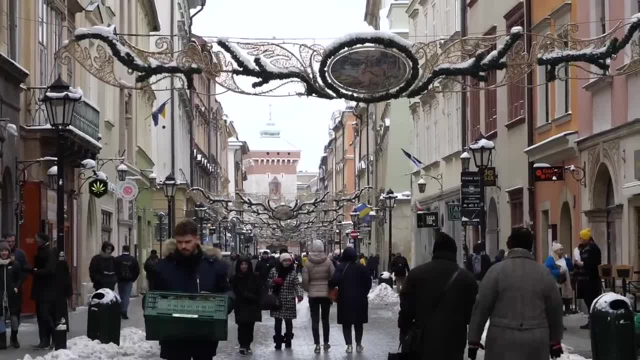 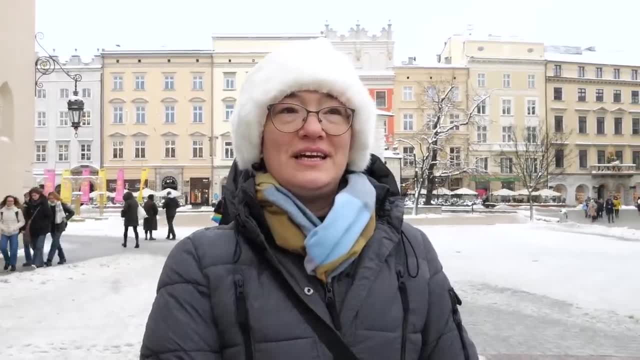 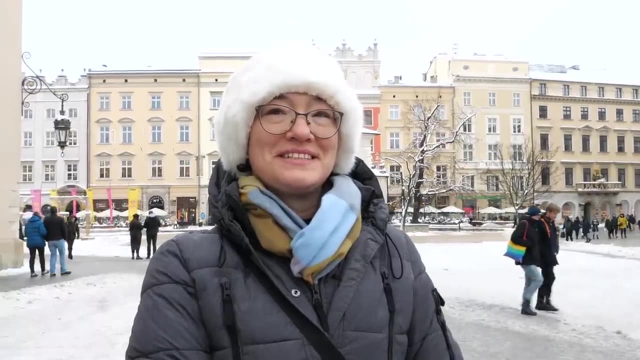 How many languages do you speak? Three. What are the three? Hebrew, English and Spanish. Wow, okay, so you're visitors to Poland. Yes, we arrived yesterday. Wow, Could you tell me in Hebrew what you think about Poland? 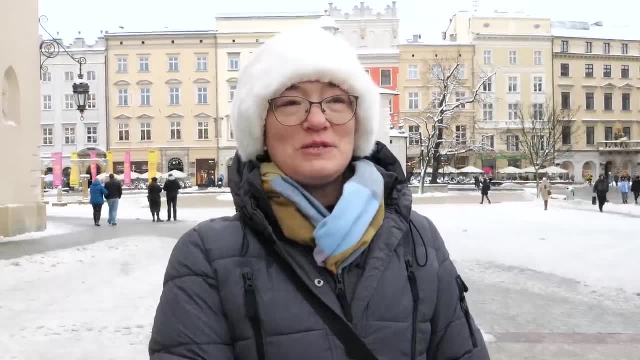 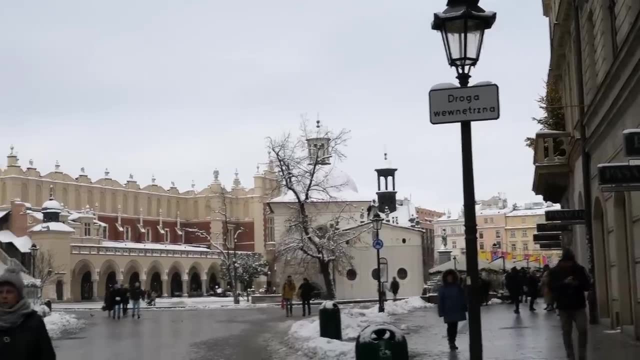 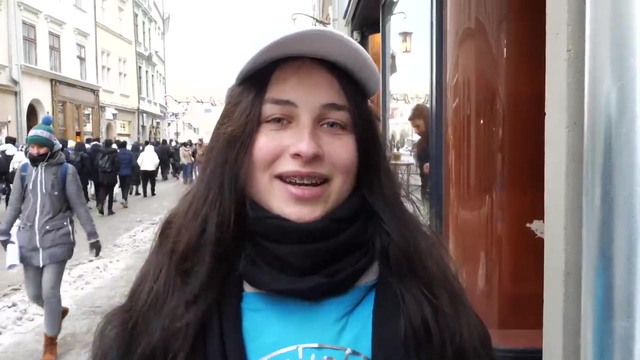 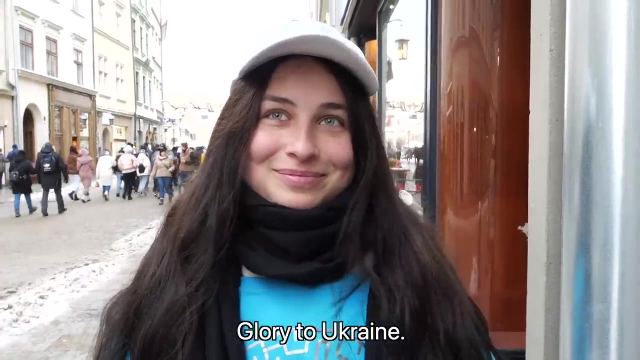 I said, Poland is a really, really nice country. How many languages do you speak? I speak Ukrainian, Russian, English and Polish. Wow, where are you from Ukraine, Slava, Ukrainian. Hello, I'm Slava. Okay, let's go left to right. 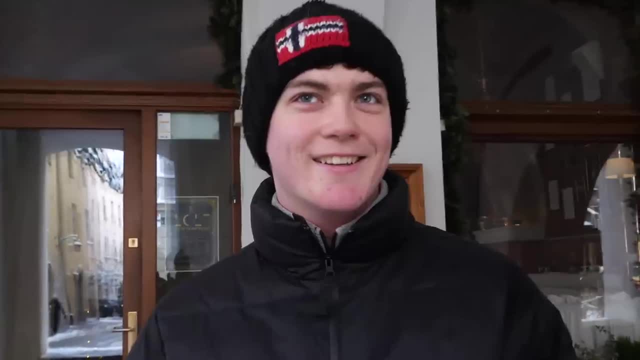 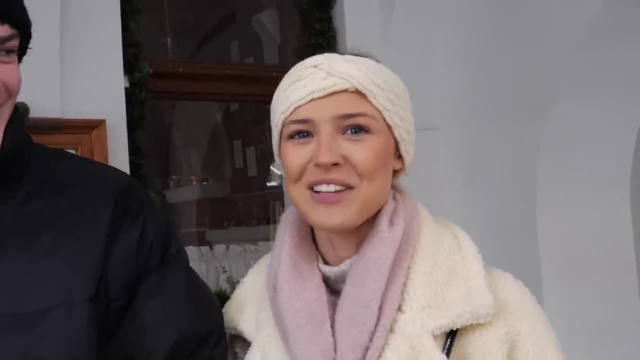 How many languages do you speak? One, What's the one? English, And where are you from Scotland? Scotland, cool, And I'm the same. Same. I only speak English. yeah, from Scotland, Cool. What do you think about Krakow? It's amazing. 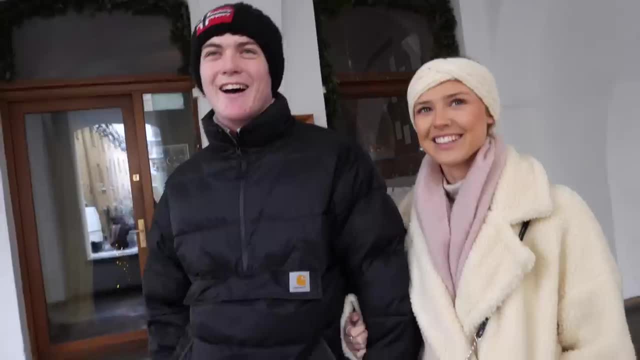 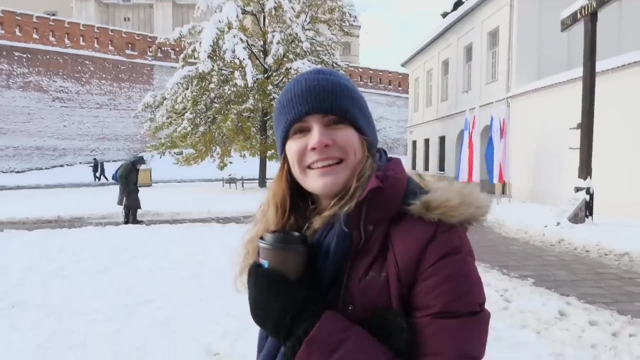 It's beautiful, Amazing, Cool. I thought you might have been Norwegian. No, not at all. Yeah, no, it's just that bad, Cool. Okay, well, have a great day, Thank you. What's your name? Ellen? 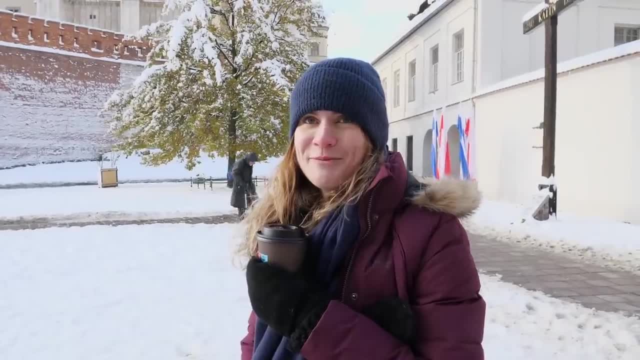 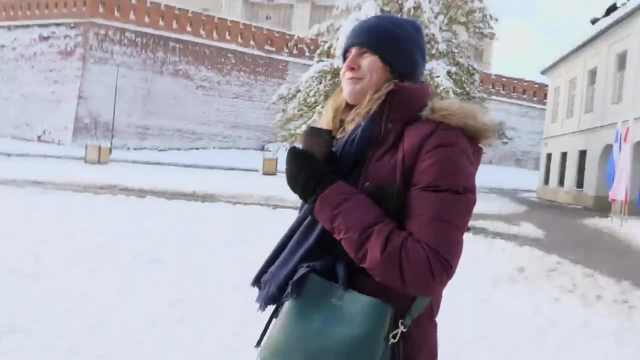 Ellen, how many languages do you speak? One And where are you from? England, Perfect, Thank you. Have a great day. It's actually pretty disgusting- We were discussing it the other day, Because obviously I speak English, Yeah. 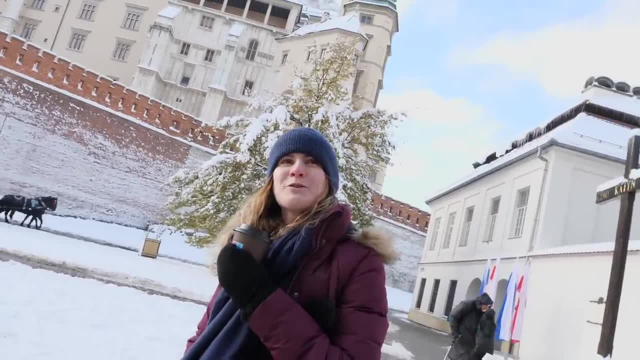 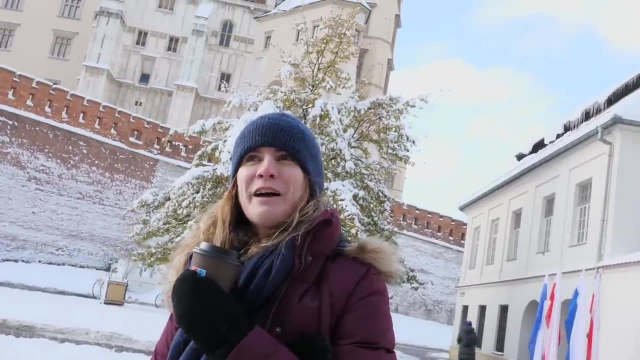 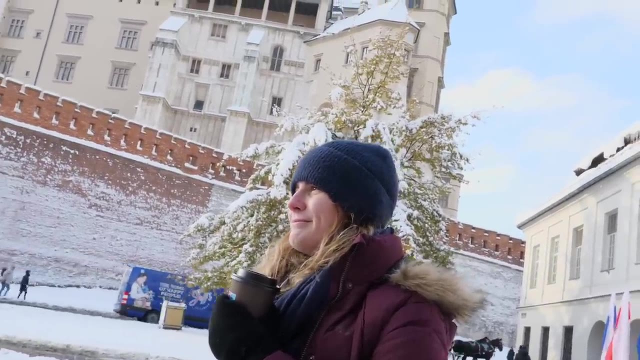 And you go everywhere just expecting everyone to speak English. Yeah, I'm Canadian, I know it's, You just expect it. It's like everybody else doesn't actually have that kind of. They grew up having to learn English And we're almost maybe naive to the fact that we can just go anywhere and just everyone will speak English. 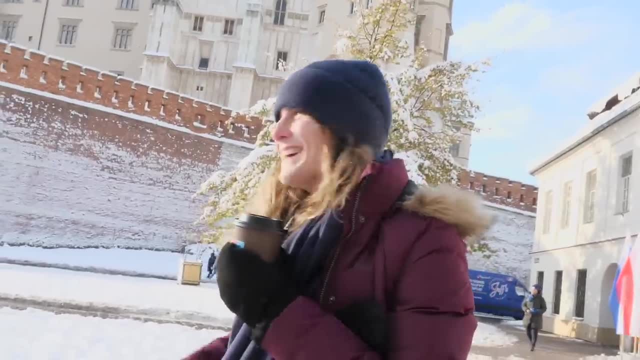 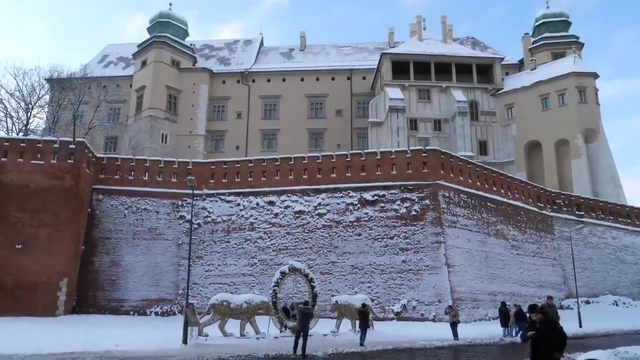 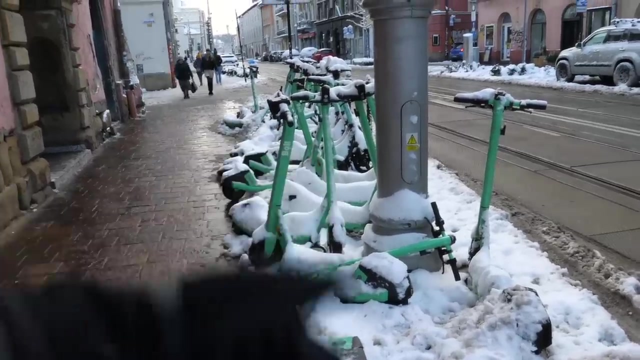 Yeah, and when you try to learn people just switch. They switch to English. Yeah, It's like, oh, she's English. Okay, well, have a great day, Take care and you Thanks. Look at this Modern-day trash. Look at all these scooters in the snow. 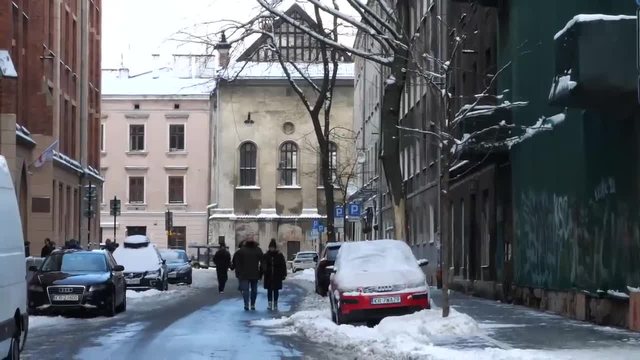 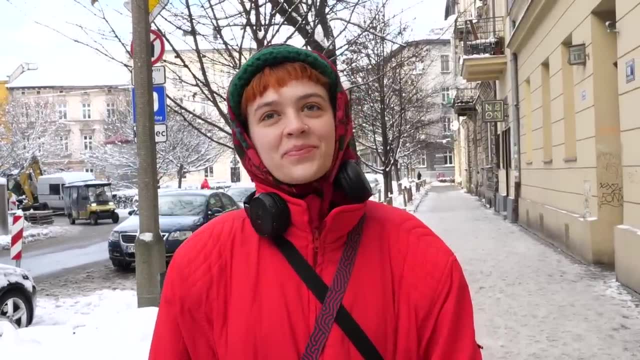 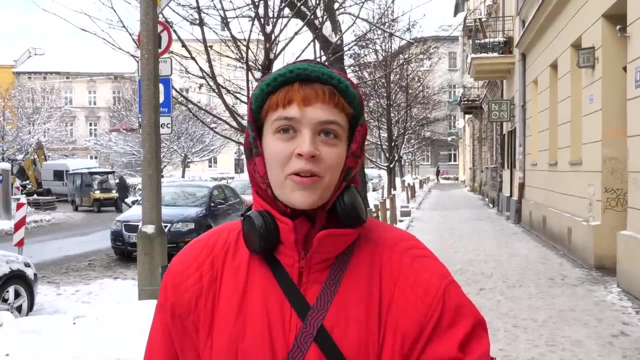 Incredible. What's your name? It's Carol- And how many languages do you speak? Right now, I'm speaking just mostly Polish and English, because I work at a cafe at Kazimierz, So it's like equally used languages in my work. 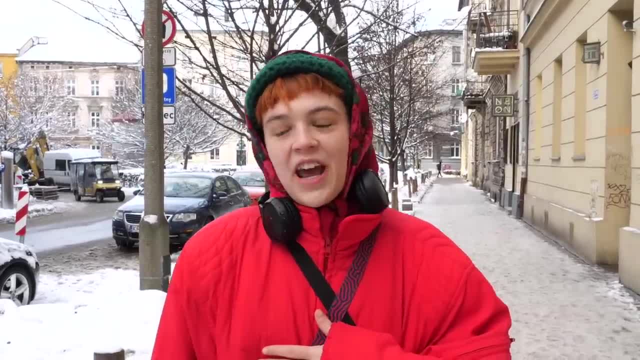 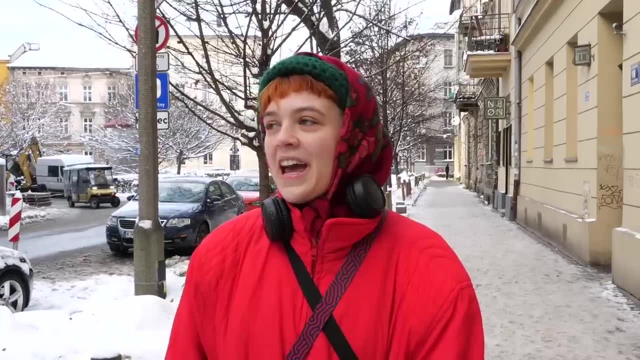 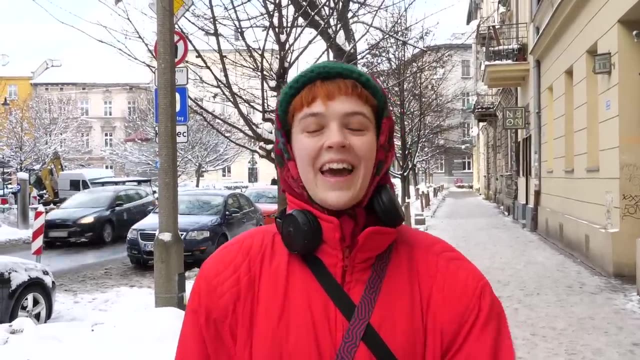 Yeah, Because of tourists. But I'm learning French, My sister is learning Japanese, So I picked up a few words And I'm planning to learn some Yiddish as well. Some Yiddish as well, Oh cool, I always dreamed about that. 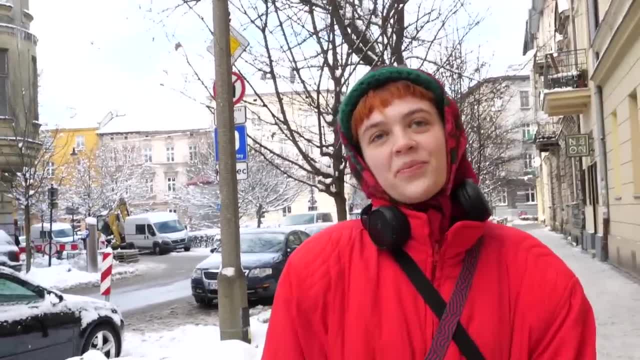 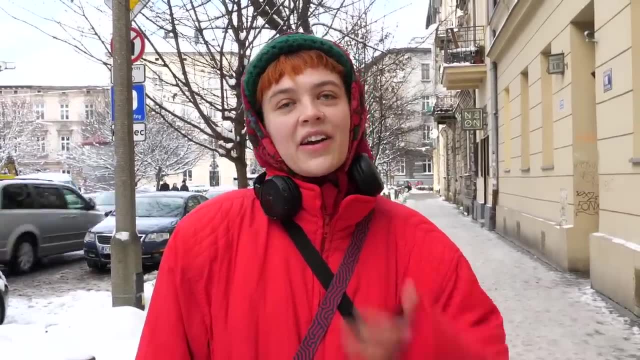 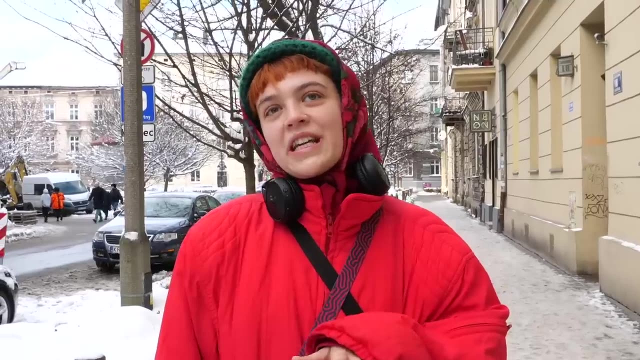 Incredible. Yeah, Just because there is like Jewish history to the city. I've always been fascinated by Jewish history And I come from a city- not Krakow, but a smaller city- that had a great Jewish minority before the war. 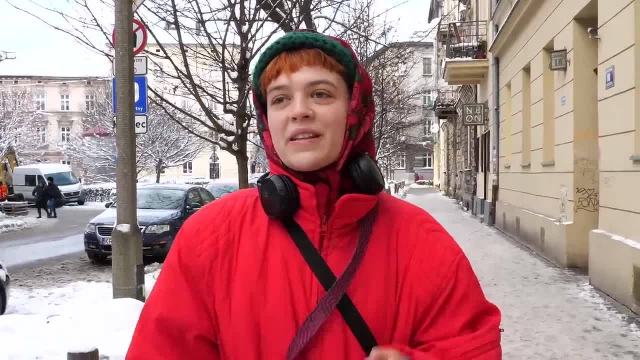 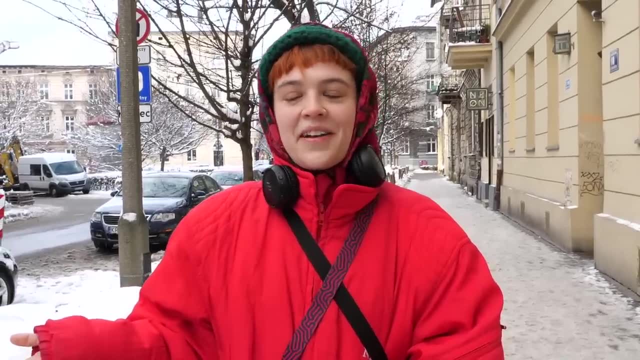 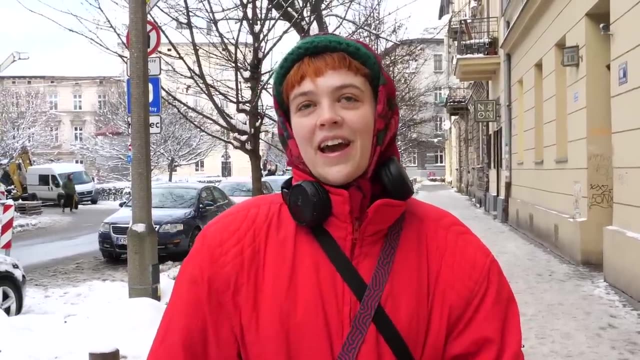 So the history of Jewish people has always been close. It always resonated with me And because I live on Kazimierz now, I would like to feel more connected to it. I think I'm not Jewish myself, but I think in Poland we should do a little bit of work in like. 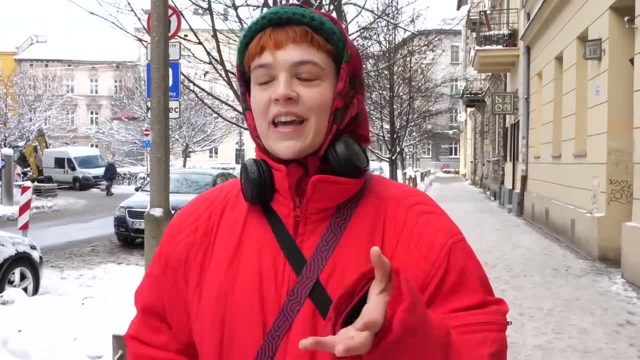 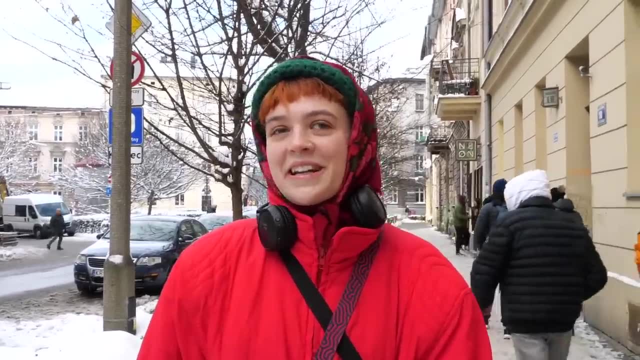 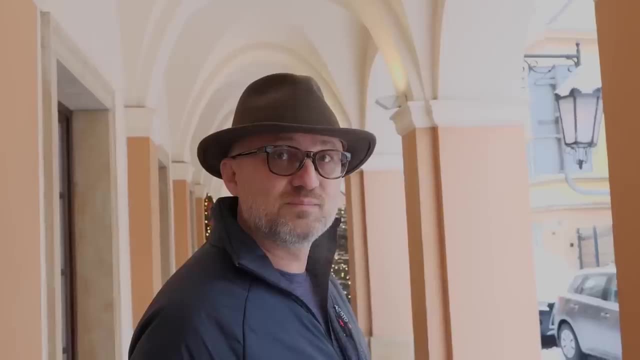 continuing the history because we existed, like these two nationalities, together for so many years. Oh, that's beautiful. Yeah, Yeah, Yeah Yeah. How many languages do you speak Besides my current one, which is Romanian? I speak English and French. 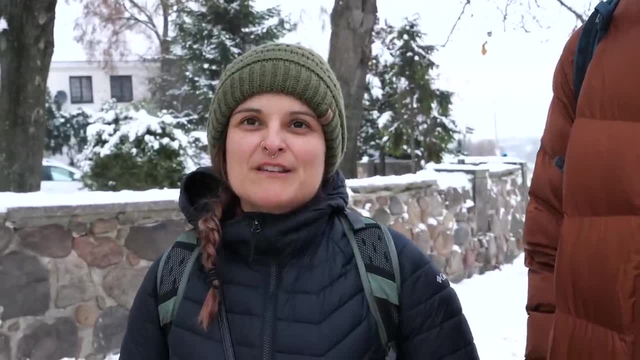 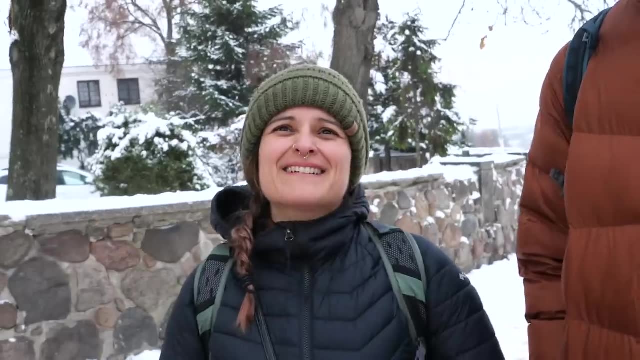 How many languages do you speak? Two, What are the two? Spanish and English? Are you from Spain? I'm from Mexico, From Mexico. Ah, Viva Mexico. Yes, What do you think about Poland? It's nice, It's very clean. 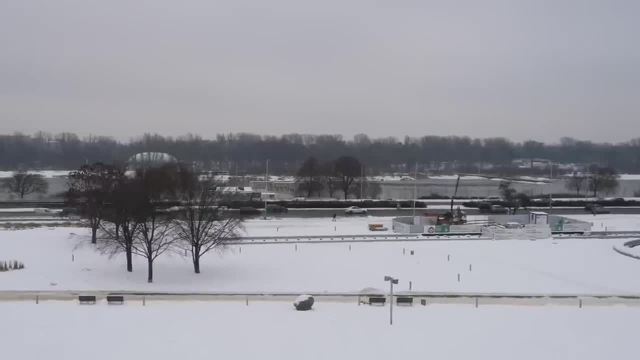 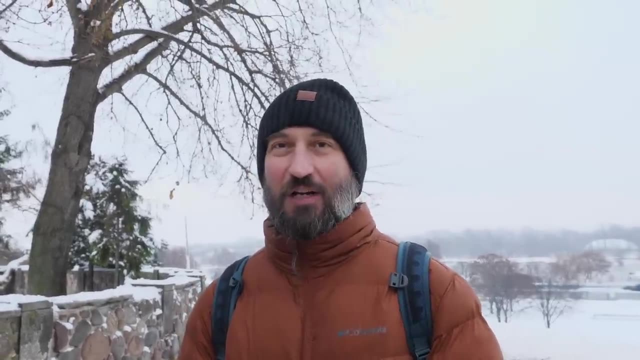 And it's very cold. Awesome. And how many languages do you speak? One And one, Canadian, Okay, One And one kind of badly, Just a little bit of German, but, of course, English. I'm from the States. 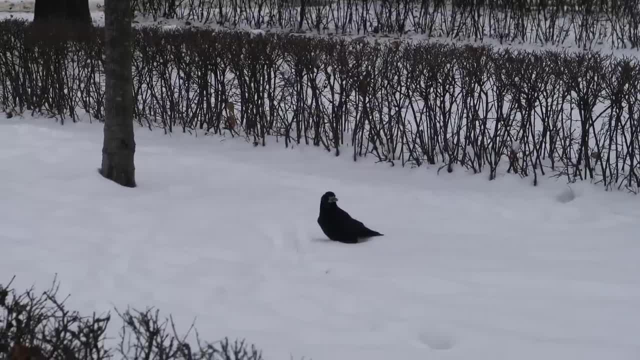 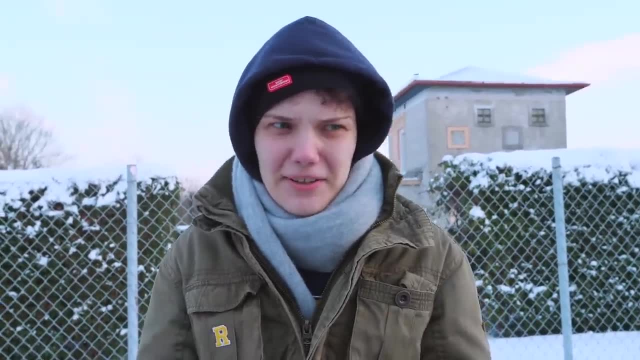 I just got to Poland today wandering around. It's been nice so far. Enjoy it. I normally say I don't speak any language very well. you know Polish and English, But I also learned French, Spanish, Russian, Japanese. 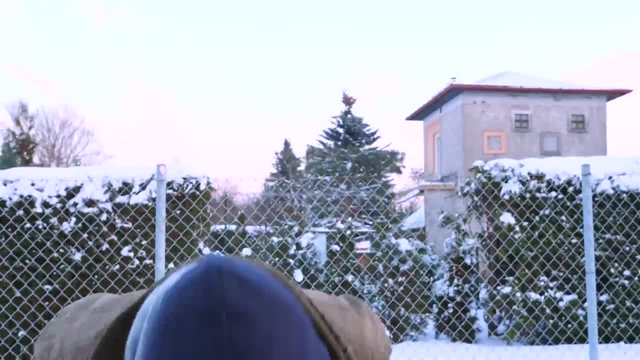 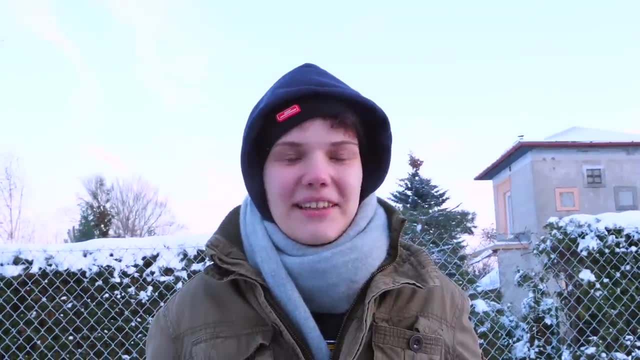 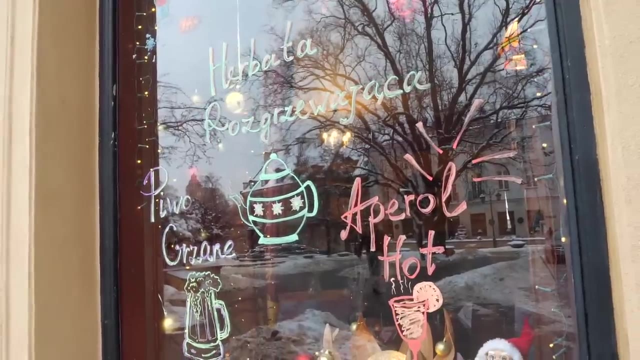 Could you throw some expression in Japanese out for the camera? What does that mean? I just? What does that mean? I just said something like. I just said something like wow, wow, that's difficult. So Polish is my native and Spanish and English. 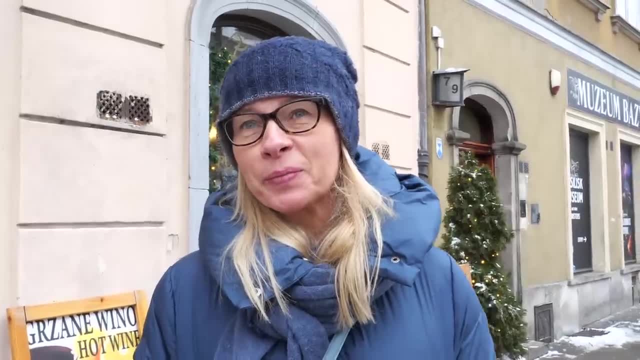 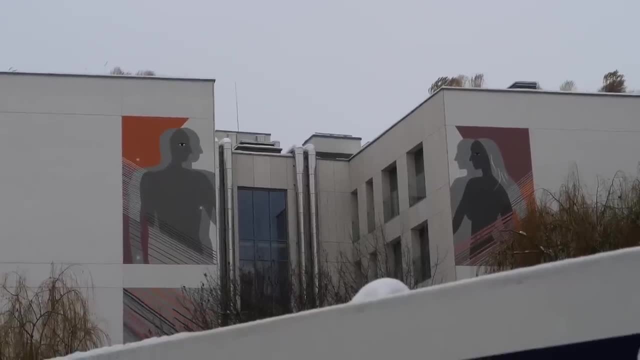 And basic Russian, really basic, Amazing. Thank you so much. Thank you, Have a good day, Good luck. Okay, What's your name? Joachim, Joachim, Joachim, Joachim, Joachim. 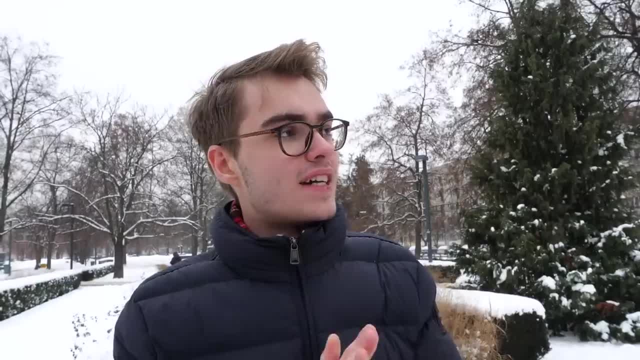 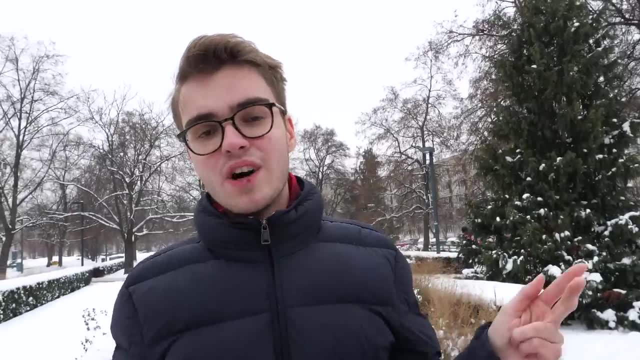 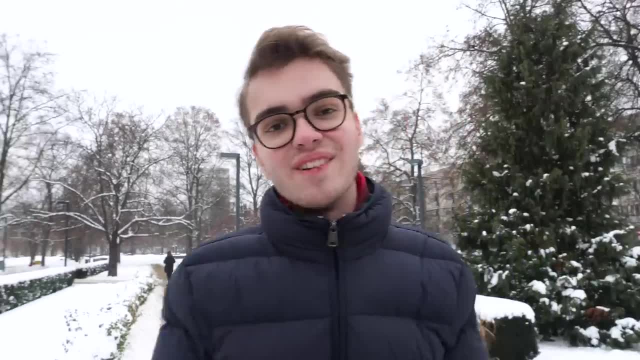 Joachim, Joachim. So Joachim is Joachim from Joachim. And how many languages do you speak? Well, fluently, I speak Polish English and semi-Hispanic Spanish, you know. 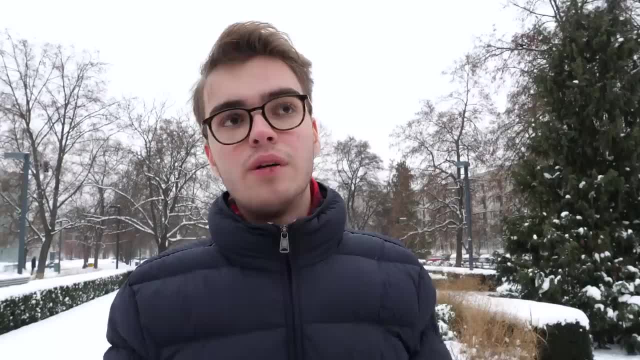 But, as all all my life, I teach myself German, but it's too complicated for me, unfortunately, So it's only English, Spanish and Polish. So Spanish it's easier than German. Yeah, Much easier and nicer, you know. 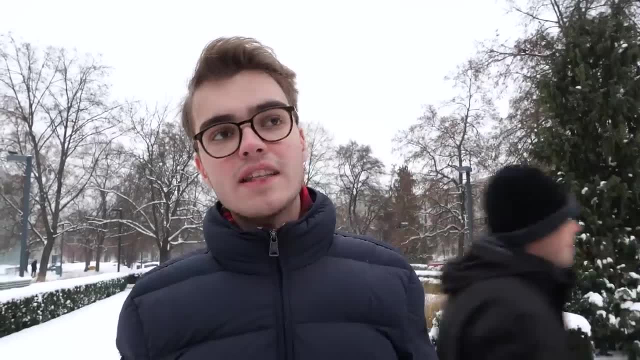 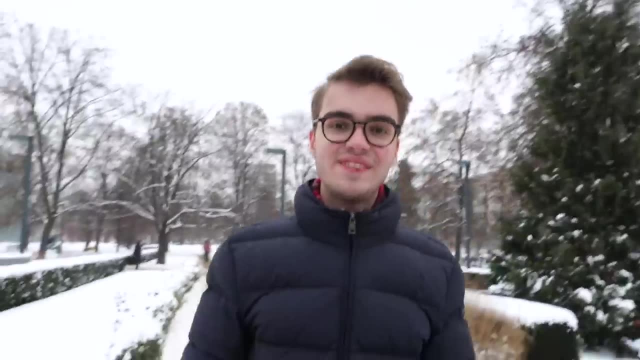 Easier to communicate with, and i'm a lot, i'm a lot, i'm a lot in spain, so vacation place, so you know, just to speak with people, with women, helps. yeah, that's all how much you give. no money, only a smile, only a smile. how? 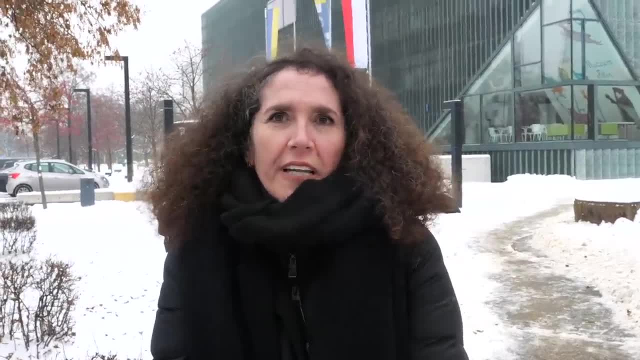 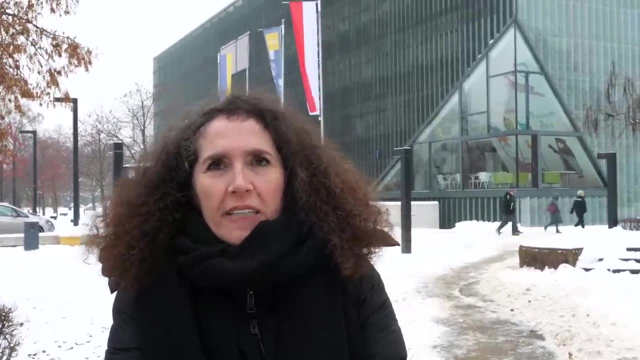 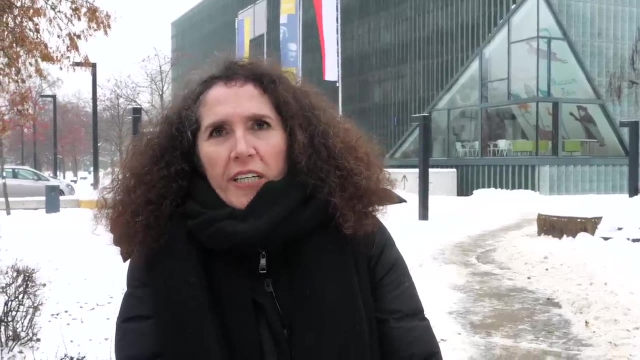 many languages do you speak? okay, i speak two and a half languages. what are the two and what's the half? the half is english. it's not so good, uh, but i speak. yeah, my mother language is turkish and german- both. ah, very cool. i was born in turkey, but i live in germany, so, uh, i live there. 46. 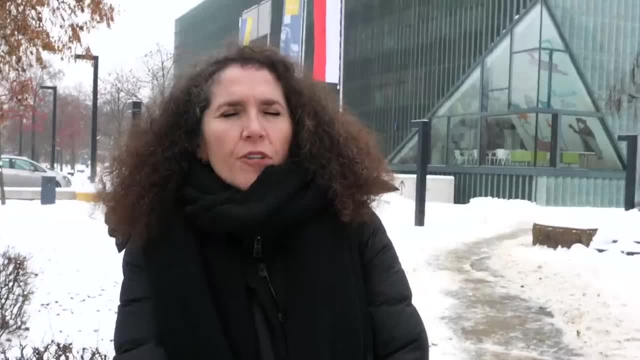 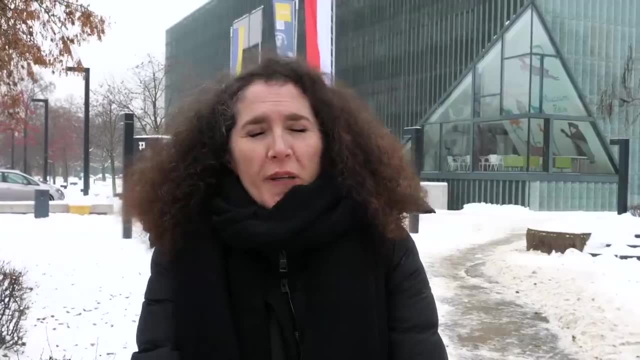 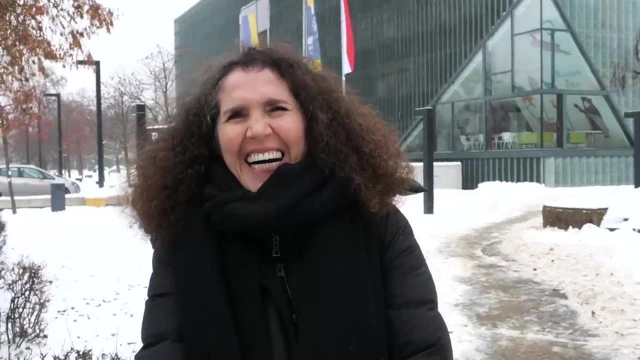 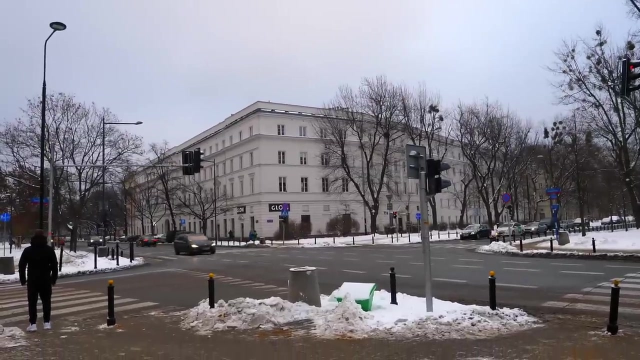 yes, and now you are visiting poland. yeah, i'm here for three or four days. could you tell me in turkish what do you think about warsaw, first of all? uh, and what does that mean? what's happening? warsaw, warsaw. it's better that i think there is lots of trees and it's so yeah. 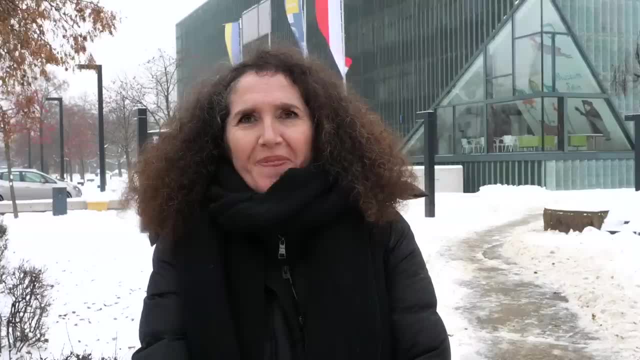 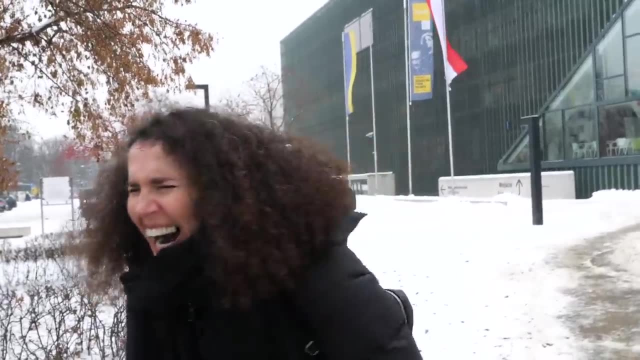 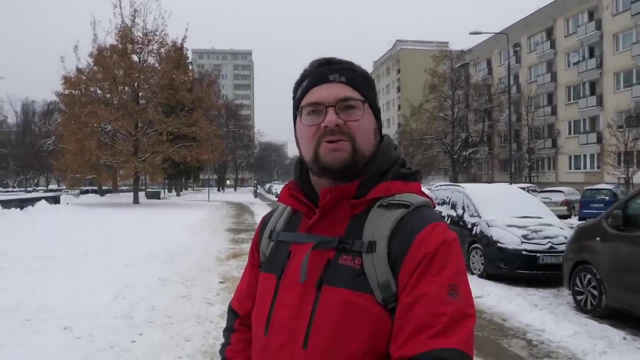 how can i say it's so beautiful, amazing, amazing, yeah, wow, thank you for your time. i appreciate it. now i learn italian, okay. so two and a half, almost three, maybe not three. three and a half, okay. how many languages do you speak? uh, two languages i speak. 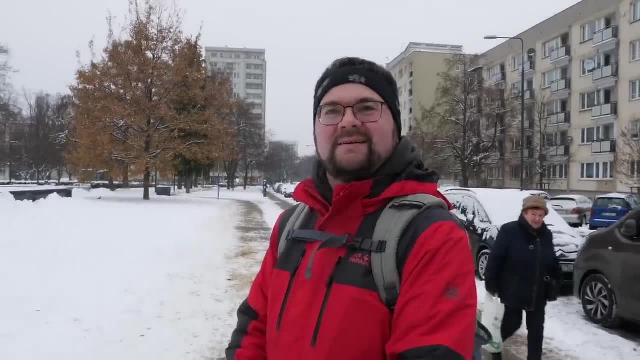 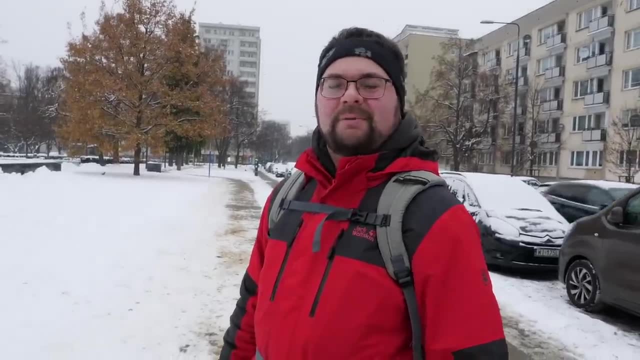 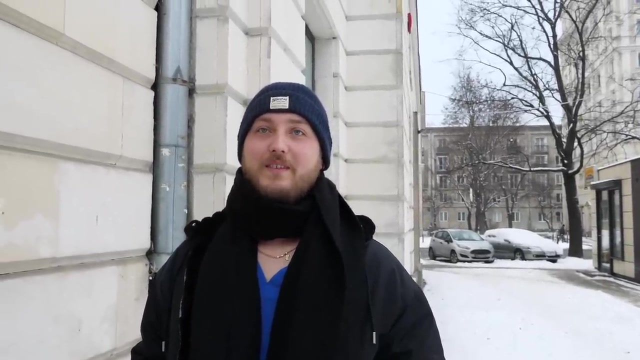 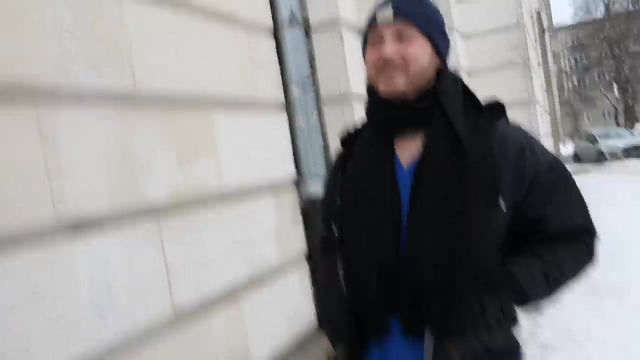 poland and germany. hi, are you from germany? i'm from germany, yes. and what do you think about warsaw? um, until now, it's very cold, but, um, it's nice. um, but cold, very cold. how many languages do you speak? two languages, what are the two? what, what, what two? polish and english. perfect, would you like to? no, i.